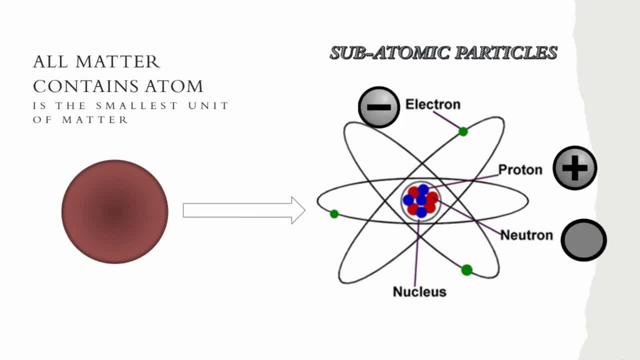 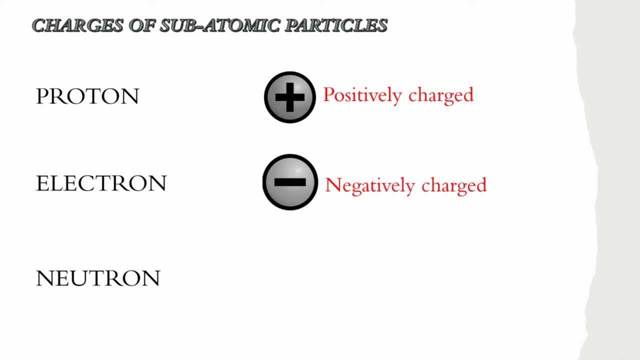 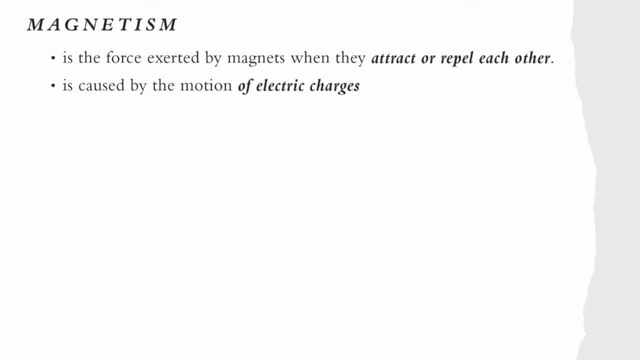 and neutron. Electron has negative charge, Proton has a positive charge, While neutron is no charge or neutral. Remember a matter with equal amount of positive and negative charges is said to be a neutral or no charge at all. In fundamental laws of magnetism, attraction or repulsion of matters is caused by the motion. 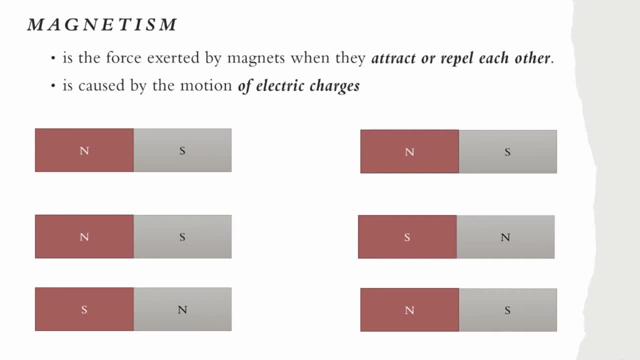 of electric charges. For example, two magnets that are facing each other with opposite poles will attract each other, Therefore they will move towards each other. Two magnets that are facing each other with the same poles will repel, Therefore they will move away from each other. This applies to electric charges. 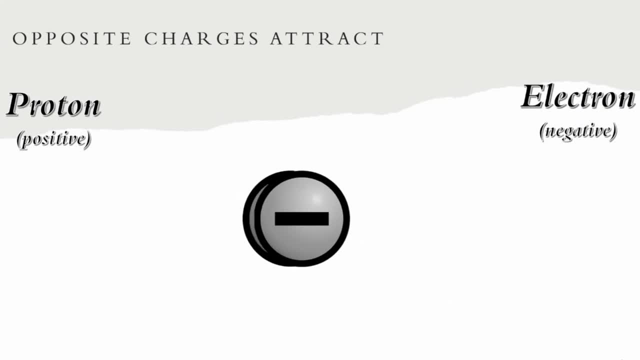 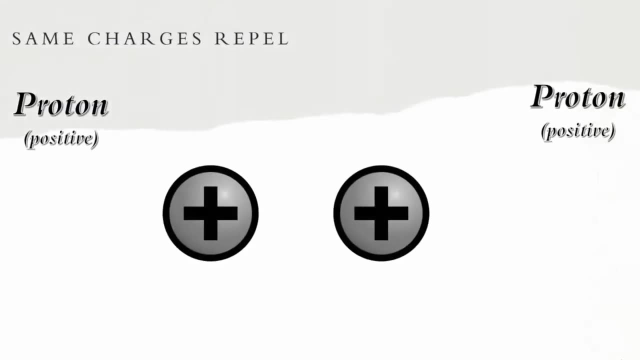 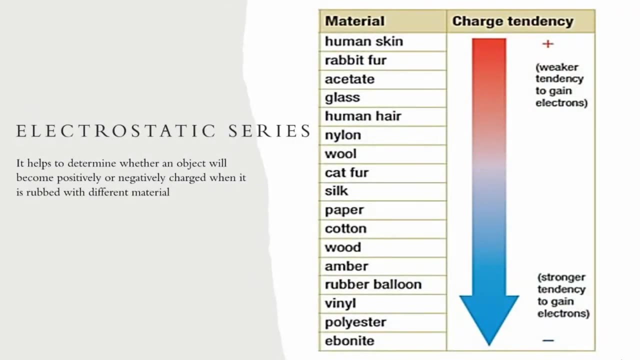 Opposite charges attract and the same charges repel. Now how do we know if an object or matter becomes positively and negatively charged? We will use electrostatic series. This is a chart that helps to determine whether an object will become positively or negatively charged. 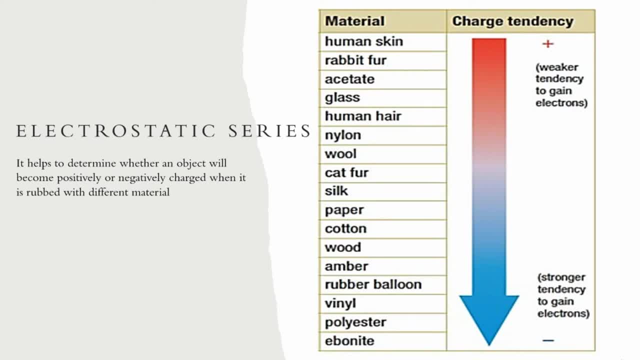 Inter zerstrich dibo Fulsag remis combustible, cestcaat, vigelous e propulsar charged. when it is rubbed with different material materials such as human hair, rabbit fur, acetate, glass hair, nylon, wood and cut fur have weak tendency to gain. 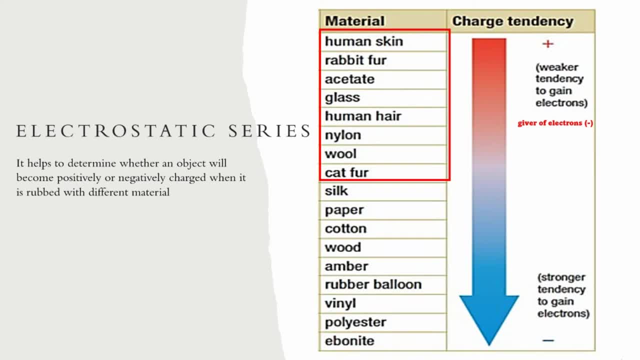 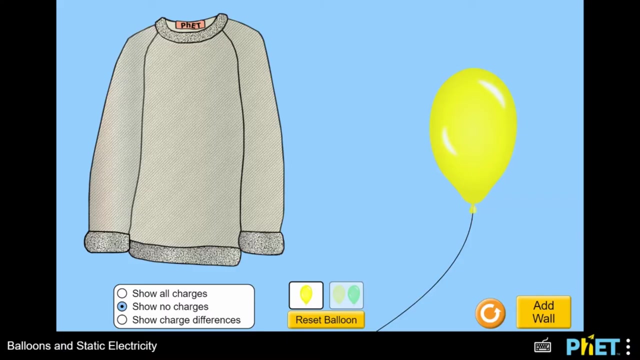 electrons. they lose their electrons to give to another object where them they made contact. below are materials such as silk paper, cotton, wood, amber, rubber, balloon, vinyl, polyester and ebonite have strongest tendency to gain electrons. they gain electrons from another object, for example the sweater and rubber. 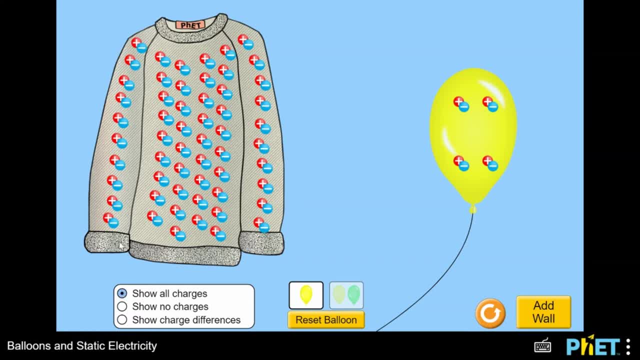 balloon initially have no electrons, but they gain electrons from another object- neutral charges- because their protons and electrons are in equal amount. now that I'm rubbing the balloon on the surface of the sweater, the balloon gains electrons and the sweater lose its electrons. the sweater that lose the 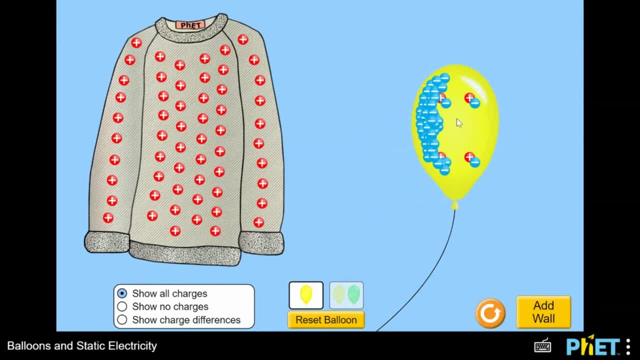 electrons becomes positively charged and the rubber balloon that gained electrons becomes negatively charged, and as I release the rubber balloon it moves closer to the sweater. this happen because the sweater and the rubber balloon have now oppositely charged that made them attracted to each other. this charging process is commonly known as 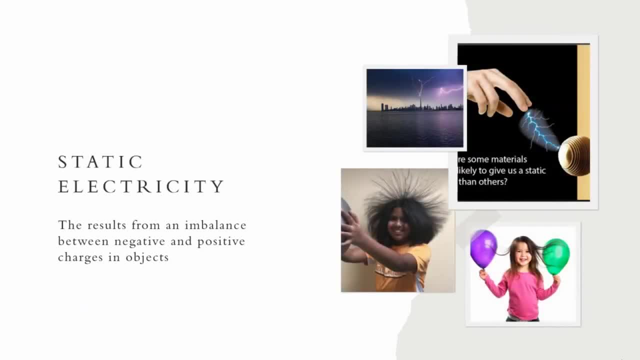 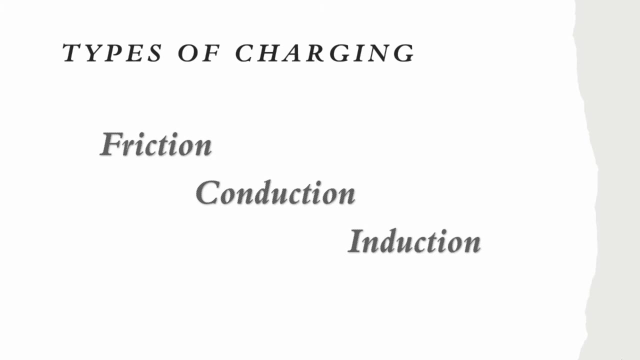 static electricity when there is an imbalance between negative and positive charges in objects. there are three types of charging process. in the sample that I showed you earlier when I rubbed the balloon against the sweater, that process of charging is known as friction. friction is the process in which a body gets 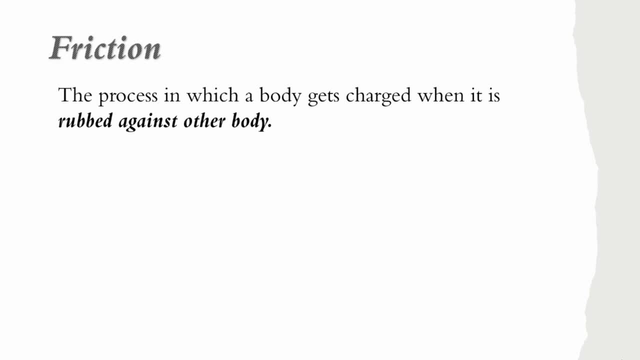 charged when it is rubbed against other body, for example. the comb and hair have initial neutral charges. but after combing your hair- which shows rubbing the hair- the comb gains electrons, so it becomes negative charge and the hair lose electrons and becomes positively charged. the hair sticks or it attracts to. 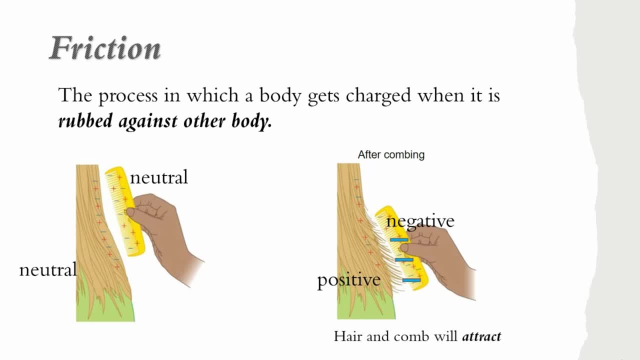 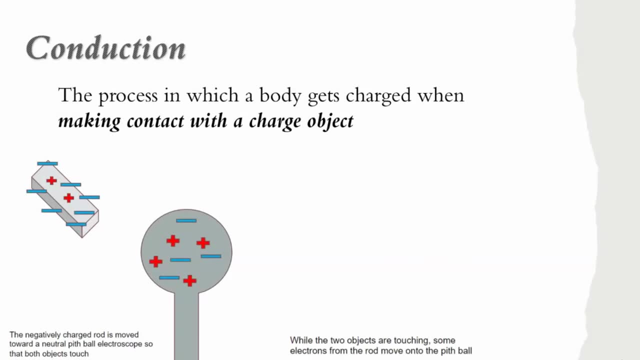 the comb because they are oppositely charged. next is conduction. conduction is the process in which a body gets charged when making contact with a charged object. if the charged object is negatively charged, electrons will move onto the neutral object. if the charged object is positively charged, electrons of the neutral object will move. 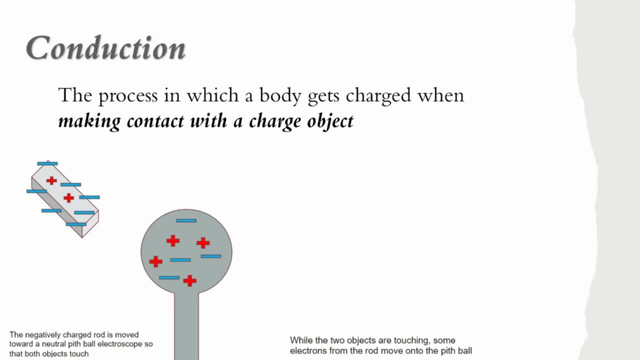 onto the positively charged object in this sample, as negatively charged rod touch a neutral piece but electroscope, some electrons from the rod moved on to the piece ball and that makes the piece ball negative charged. obviously If the charged object must move strongly the battery will move稍. tilline bullet touched: the детale comes from the duythe electric. 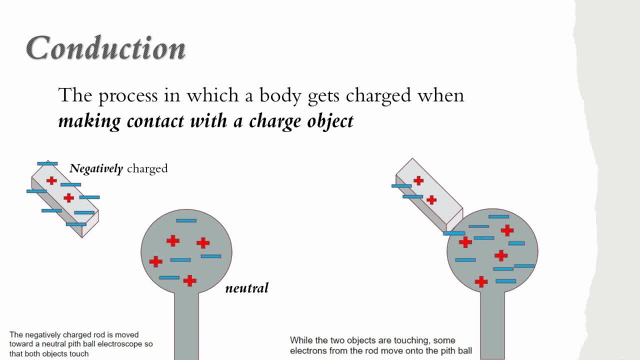 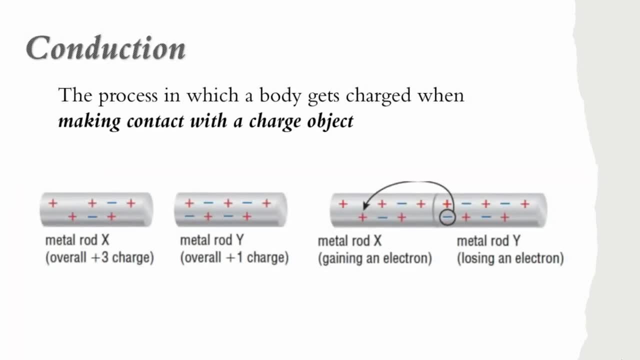 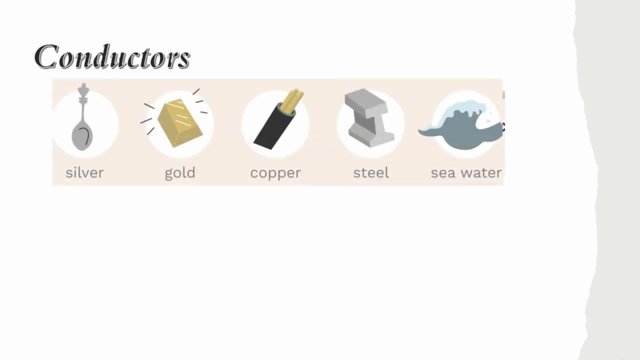 charged. if to charge object touched, electrons will move away from the object with more electrons until both objects have the same charge. materials that allow electrons to flow freely are called conductors, such as metals. on the other hand, materials that do not allow electrons to flow easily through them, 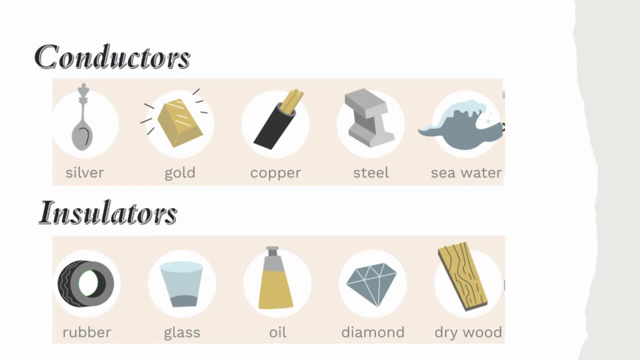 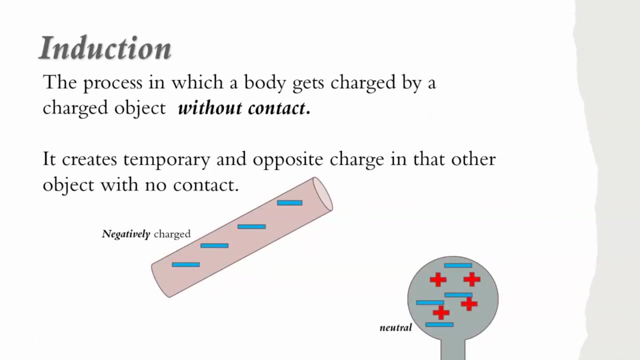 are called insulator, such as rubber, glass, plastic, oil, diamond and dry wood. and this is also the reason why electric wires have rubber coating: to prevent electricity from flowing direct to our hands and to prevent electric shock. and the third one is induction. it is the process in which body gets charged by a 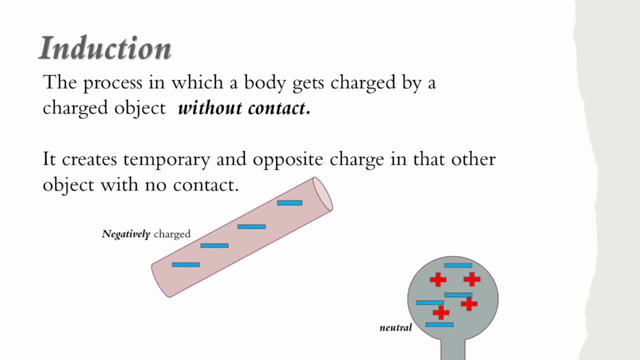 charged object without contact. it also creates temporary and opposite charge in that other object with no contact. for example, when they move this negatively charged pipe closer to the neutral charged ball, the negative charge in the ball away and makes the front size of the ball positively charged. and like what? 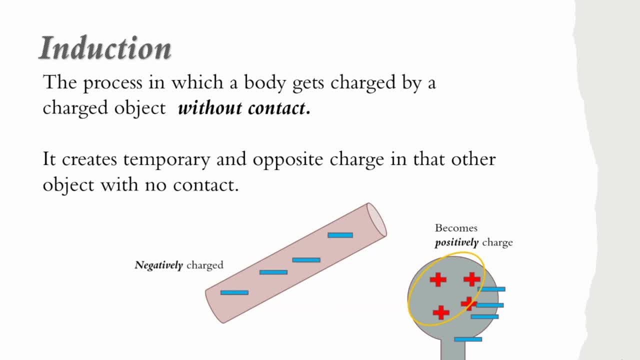 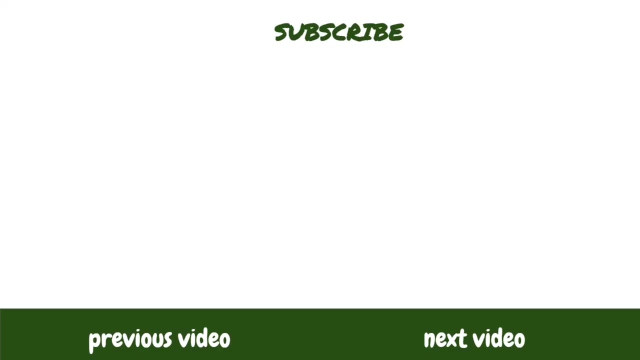 I've said, this can only happen temporarily because the negative charges did not transfer from one one object to another. alright, that's all for today. see you in our next video lesson. if you like this video, please subscribe to our channel and hit that notification icon for more videos like this. bye. 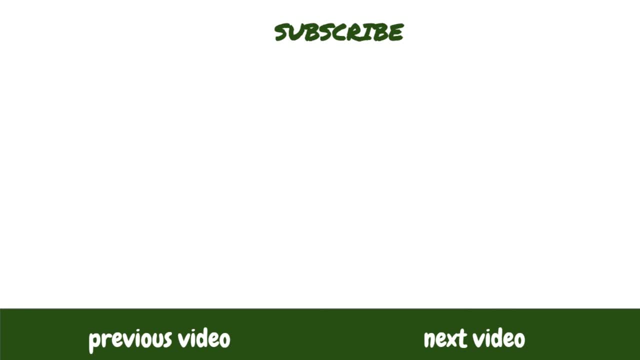 everyone and have a great day.